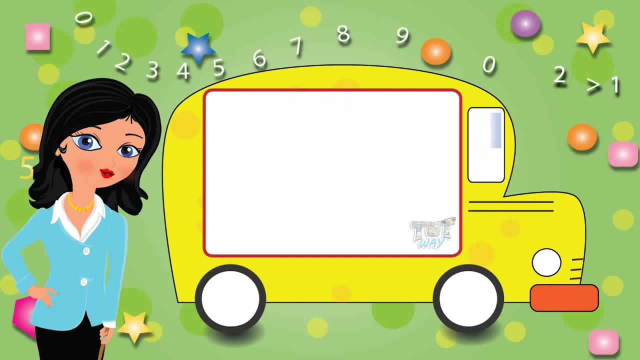 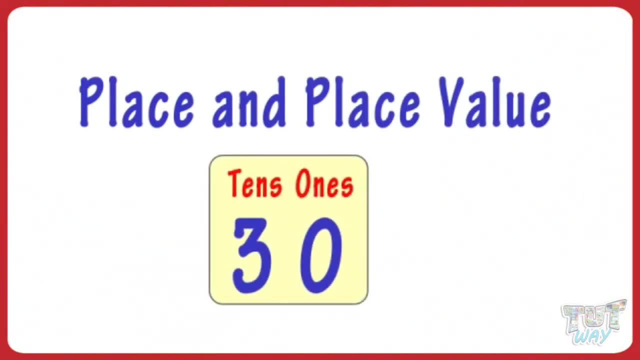 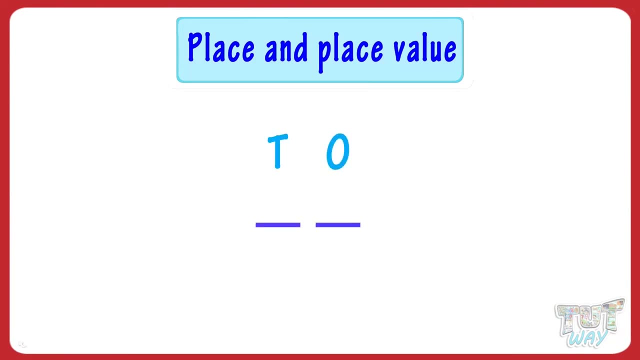 Hi kids, Today we will learn what is place and place value of a digit in a number. So let's get started. Place is the position of the digit in a number. Example: here we have a number. Place of 3 in this number is 10's place, Place value it is. 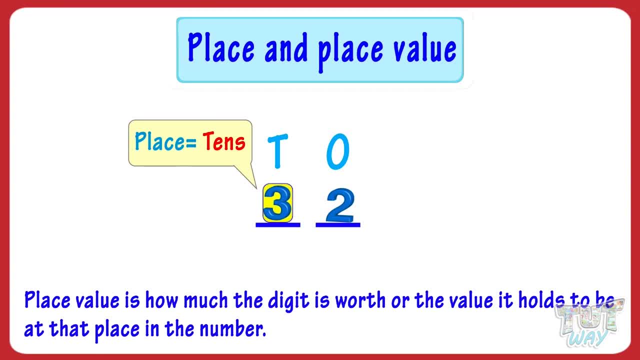 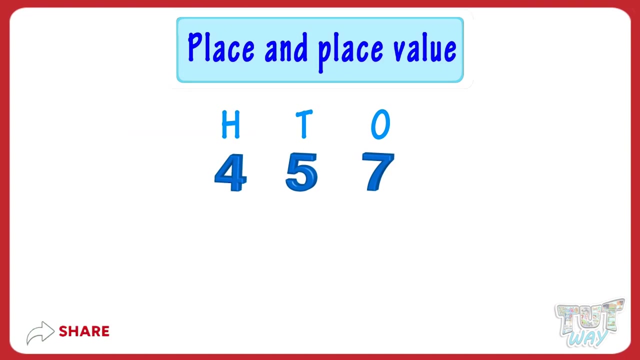 how much the digit is worth or the value it holds to be at that place in the number. Example: place value of 3 in this number is three tens or thirty. Let's learn the concept with more examples. We have a number 457.. Let's start with seven. Its place is one's place and place value is. 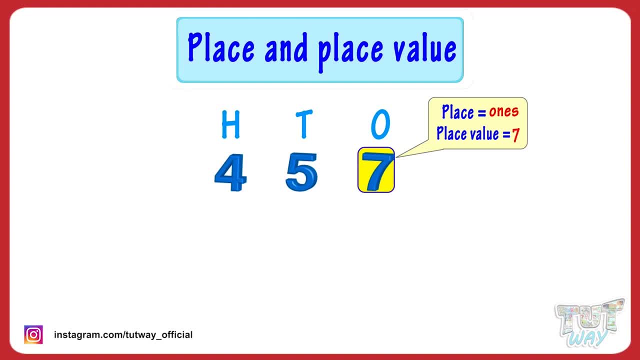 seven ones, that is seven. Place of five is tens. Place value is five tens. that is fifty. Place of four is hundreds. Place value of four is four hundred. So, kids, let's take another example. Here we have another number. Now let's see the place and place of each digit in. 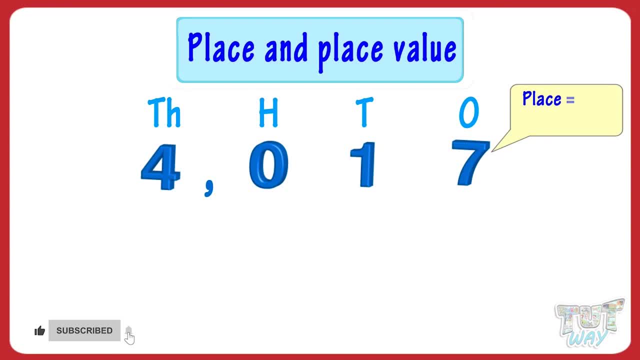 this number. Place is seven ones and place value is seven. Place of one is tens and place value is one, ten, that is ten. Place of zero is hundreds and place value is zero. hundred or zero, No matter what is the place of zero, place value of zero is always zero. Place of four is thousands. Place of 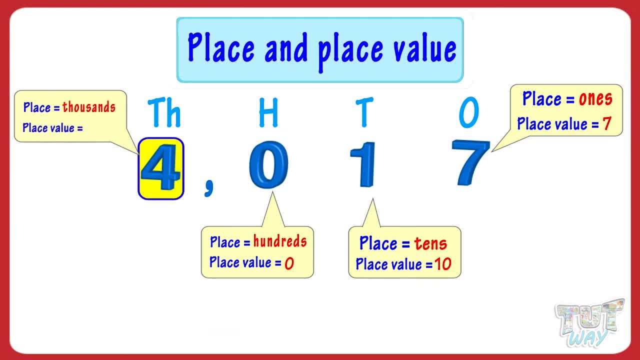 celebratory position is always two thousand, Place of one is hundreds and place value of two is hundred and place value of one is three thousand. Place value of three is dollars and place value of one is. before you raise a kulak will go from one second or Chic. 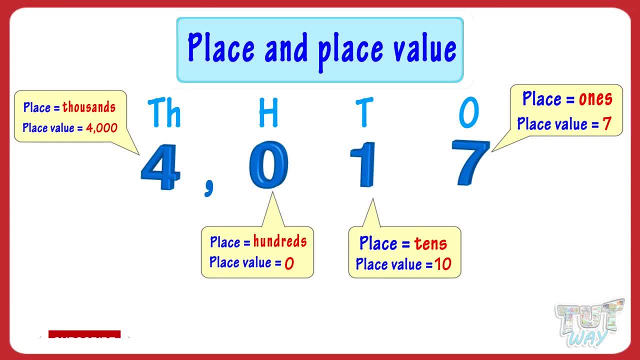 to one slash. So the logic of the box is exactly the same: Place value of five is five hundred and place value of ten is four thousand, which is about two hundred, and place and four is about four thousand. So, kids, now you have a fair idea What is place and 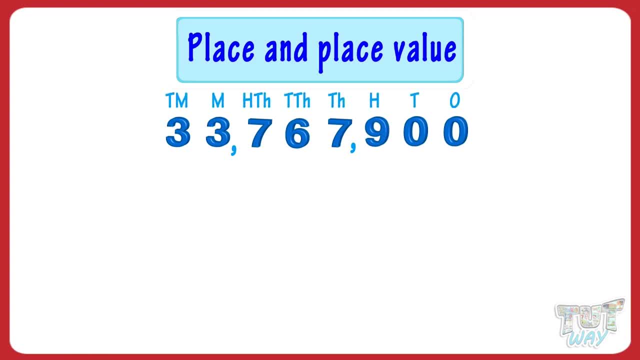 place value. Let's take one more example for practice: Kids. now we have a big number. It is thirty three million. twelve horses. This is twenty four million, always four guys. Now let's answer a few questions. Which digit is in the 10,000,000th place in this number? 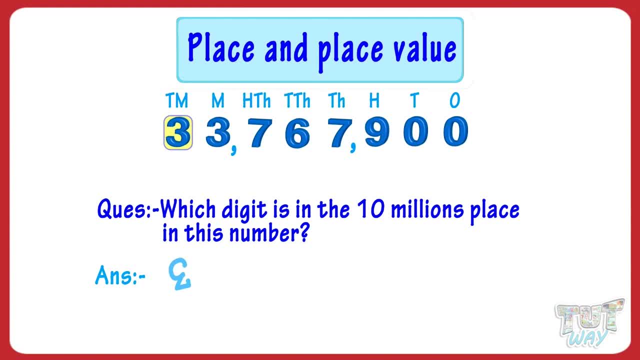 Can you answer? It is 3.. Now, what is the value of underlined digit in the number? Value of underlined digit is 60,000.. Now, what is the place of underlined digit in this number? The place of underlined digit is 10,000.. 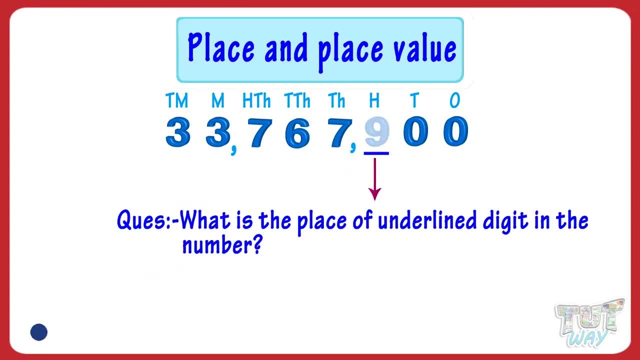 What is the place of underlined digit in the number? It is 100.. Which digit is in the 1,000,000th place in this number? 3 is there in the 1,000,000th place in this number. 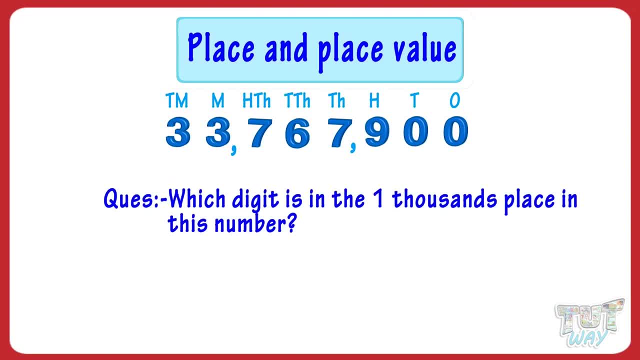 Which digit is in the 1,000,000th place in this number? 7 is there in the 1,000,000th place in the number. Now, what is the value of underlined digit in the number? It is 100.. 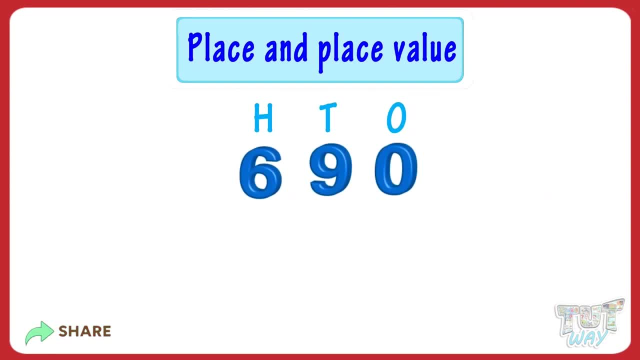 So, kids, if a digit comes more than once in a number, everywhere, it's place and place value will be different. So, kids, what have we learned today? We have learned: place is the position of the digit in a number. Place value is how much the digit is worth.